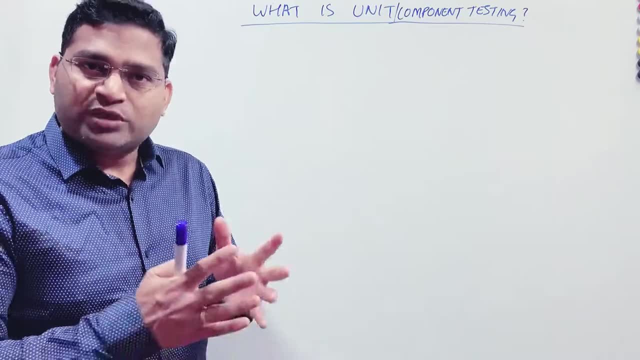 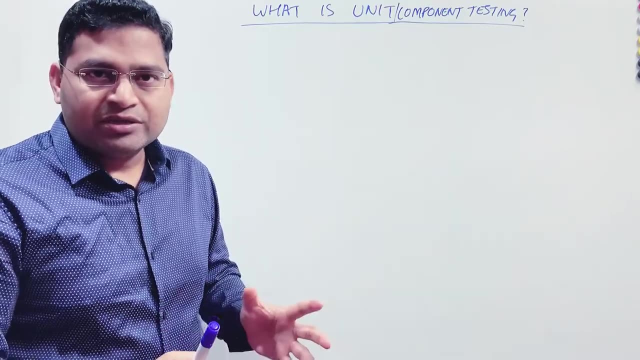 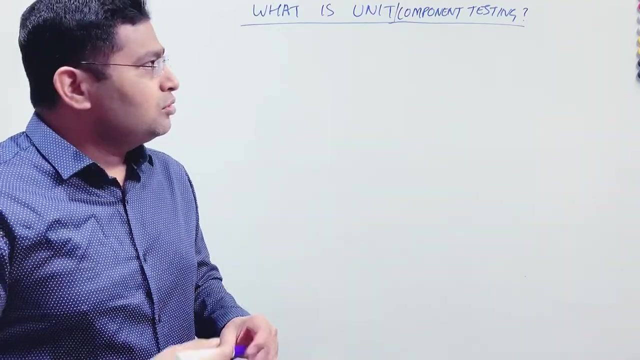 exactly, unit is right, So that is very important. if you understand the topics practically and can correlate with the real life examples out there, you will understand software testing or any development or automation, just like you know it will be a breeze. So that's what. 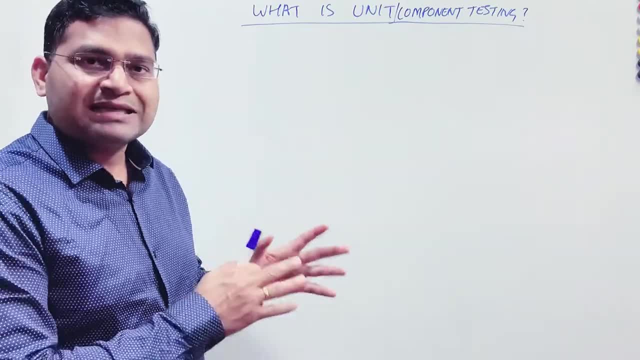 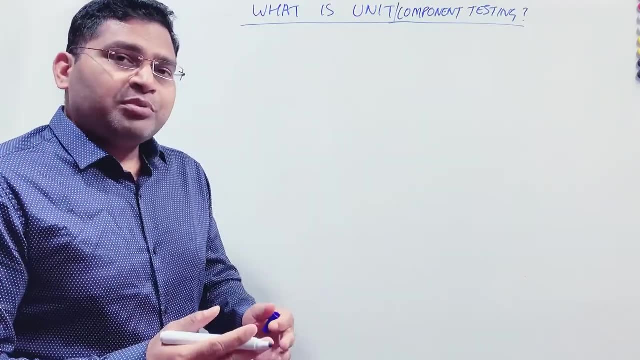 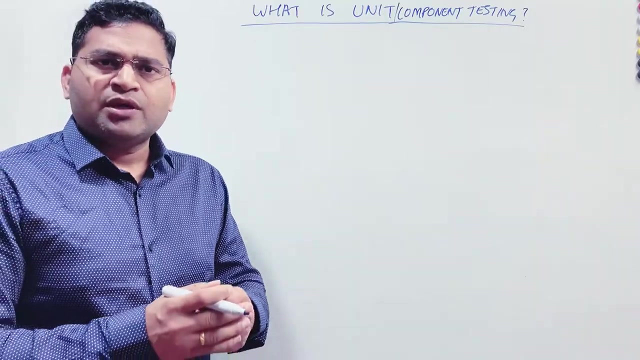 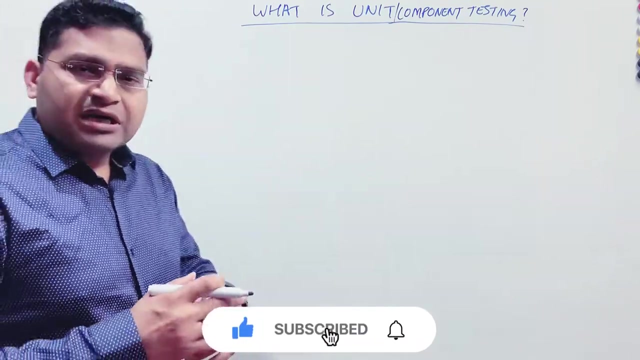 I'm trying to do here: try to simplify things as much as possible and correlate those with the real examples. all right, So let's take an example of a car manufacturing. okay, So if a company is manufacturing a car, what exactly could be a unit in the car? So give it a thought. say, for example, car will have you know. 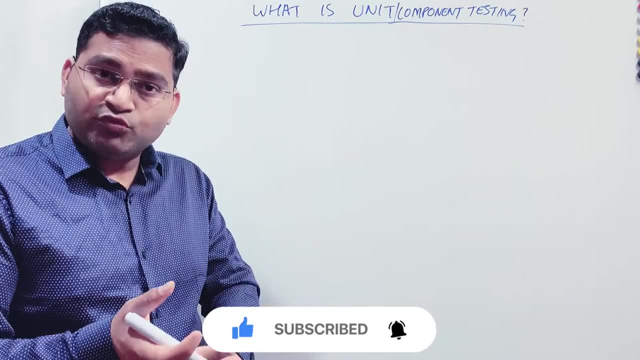 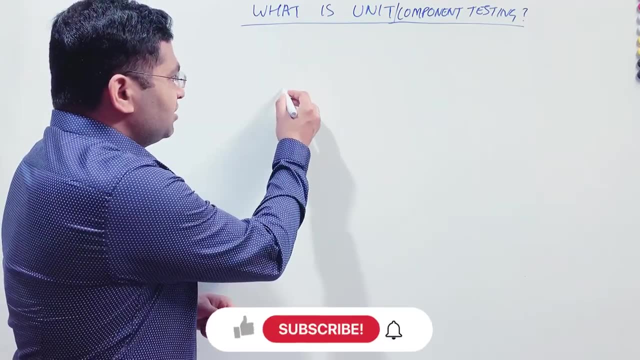 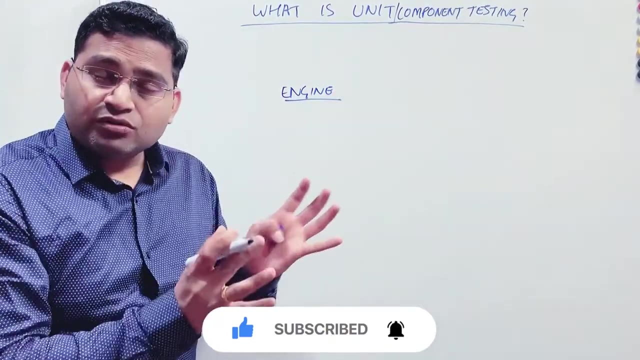 engine, four wheels, so there will be wheels, the body. but if you segregate all these parts, say, for example, engine, I'll say right, So there will be engine. So engine is not a standalone activity, right, It's not a standalone part, it's basically a combination of lots and lots of parts. 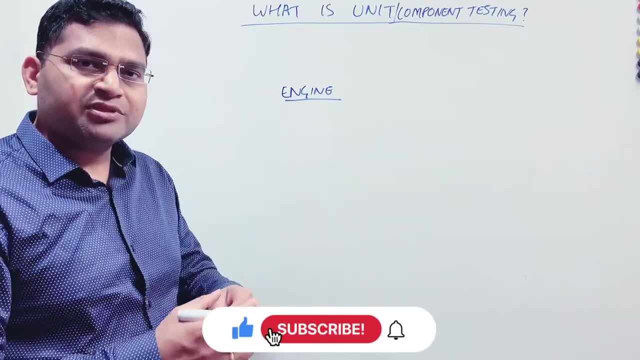 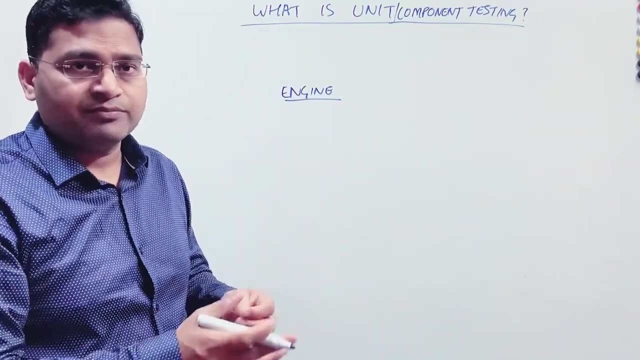 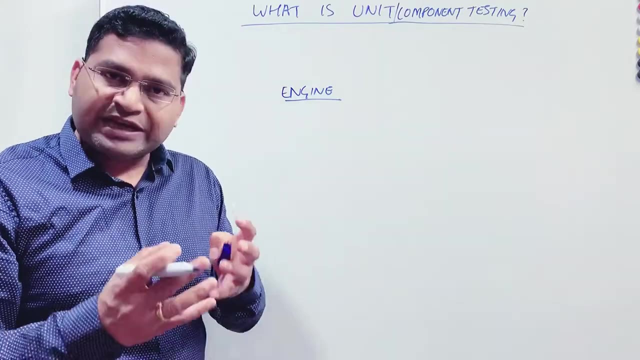 right. So there will be very small items that combine together and make the overall engine that you, that is fitted into the car, right? So if we drill down the engine and drill down to the smallest unit of that engine, this is what is called unit That can be tested independently. 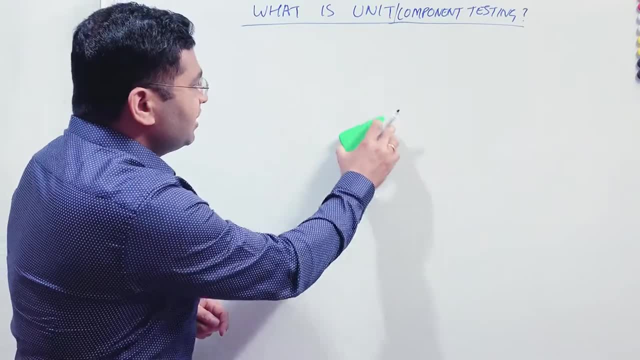 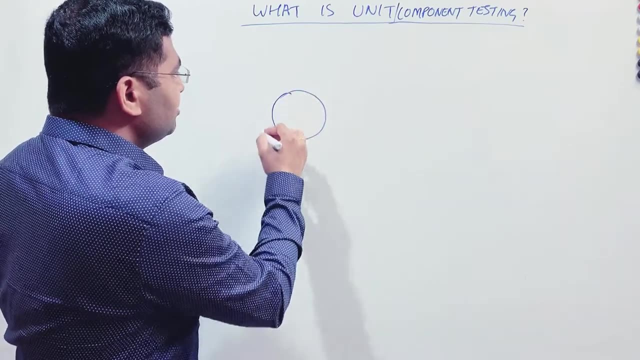 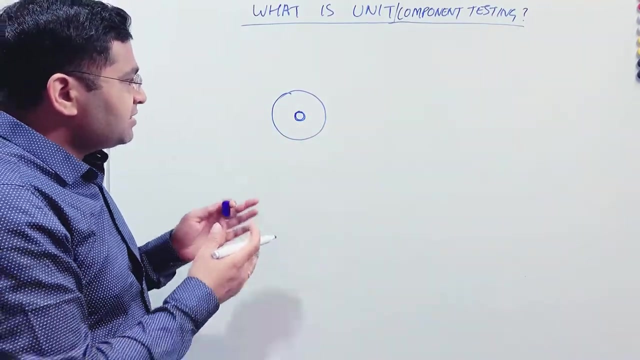 all right. Now that's the analogy of car and engine. If say, for example, I'll take an example of the tire, okay, So tire? do you think tire will be a standalone activity or a standalone unit that can be tested, or that's the smallest unit in the car? 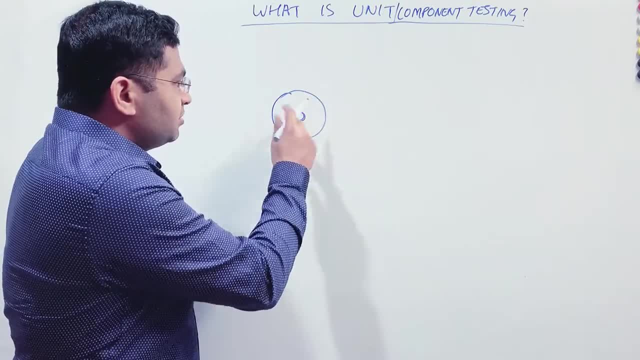 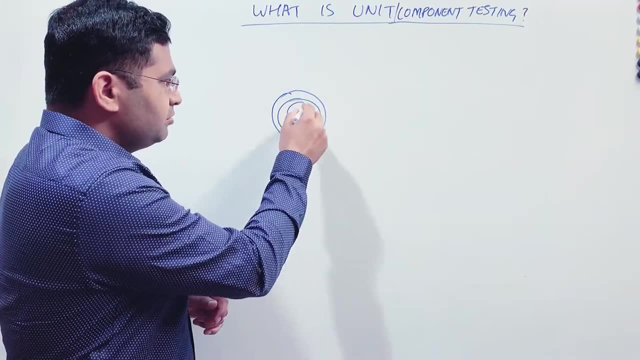 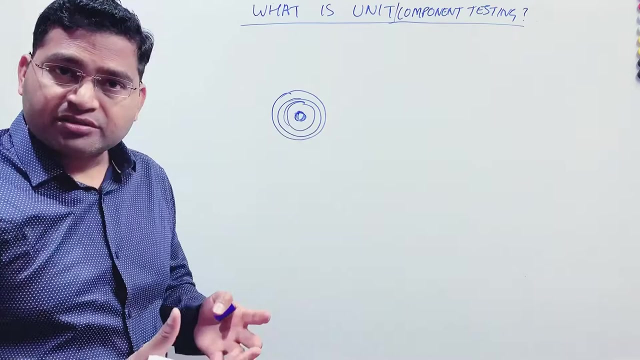 I think the tire or the wheel basically will have the tire, so tire can be tested separately. It will have the rim, the metal, you know. rim, that is another piece, another unit right. And then within the tire there are ball bearings, which are another, you know. 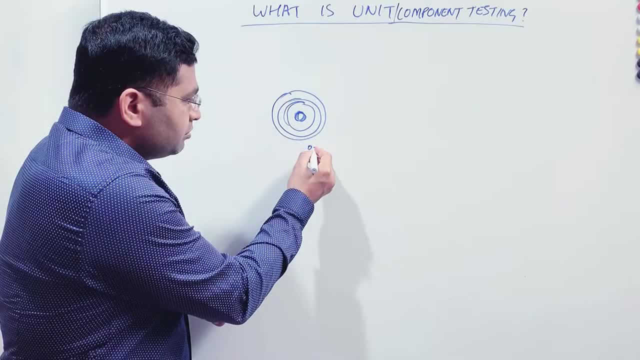 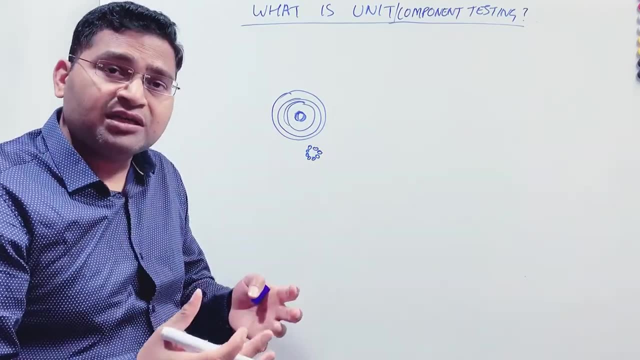 unit And within the ball bearings there are smaller, you know, rings there within the ball bearing right. So all these, the smallest item that can be tested independently within the car is a unit, if we talk about the car manufacturing right. So these are these, you know small. 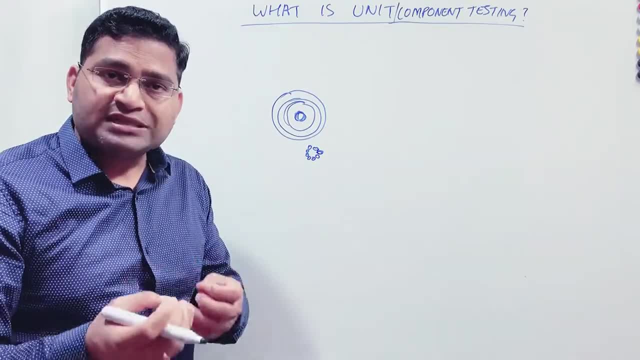 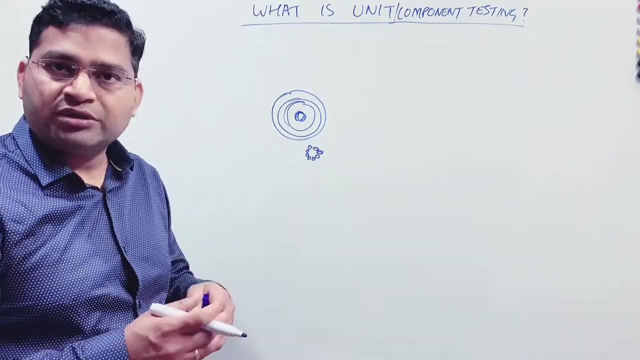 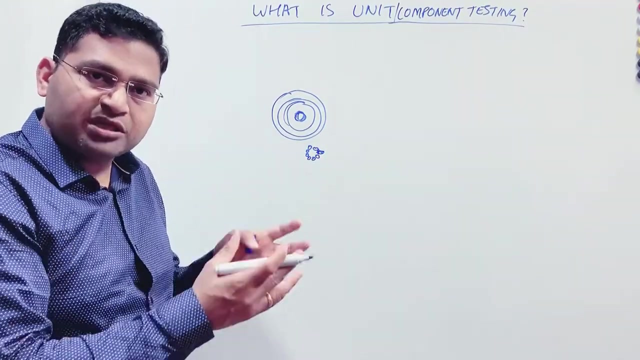 bearing units. the round units are the smallest testable part because those are tested, you know, tested to you know. see whether they are all good. the quality is good. there are no issues with those. So these are, you can say, units in the car wheel When you assemble the car wheel. 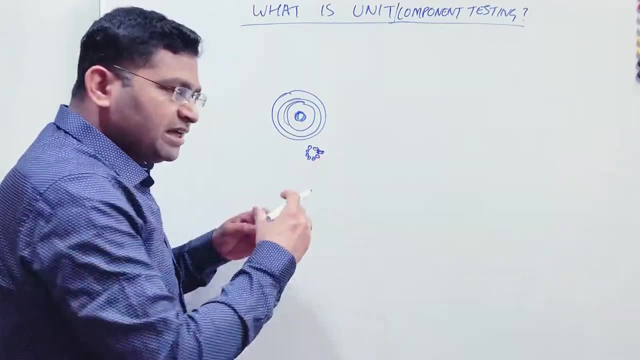 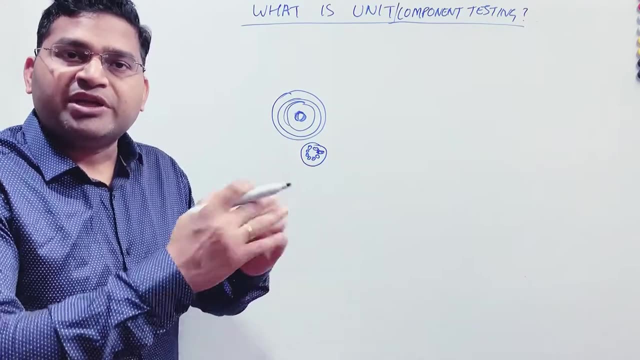 this is the unit of the ball bearing. When this is combined with the outer layer, that's another unit and these two are combined, then that becomes the bearing. okay, So this is how you can correlate unit to the actual software world. okay, 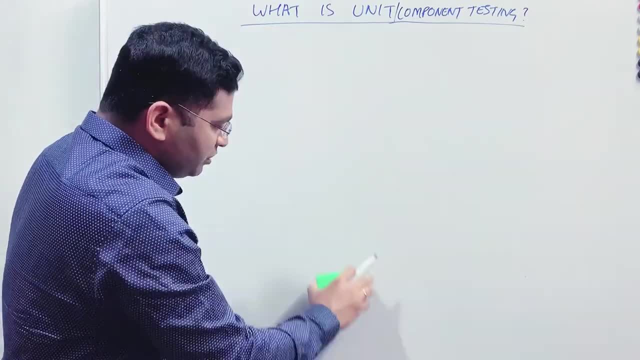 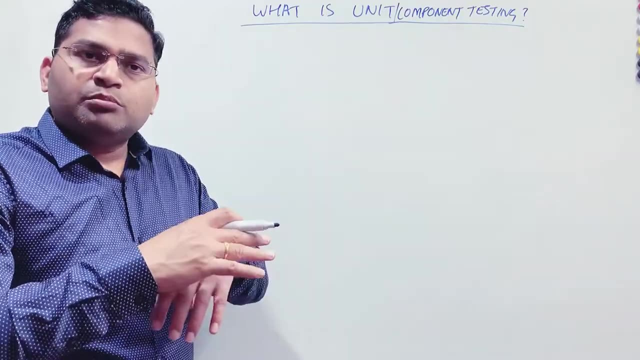 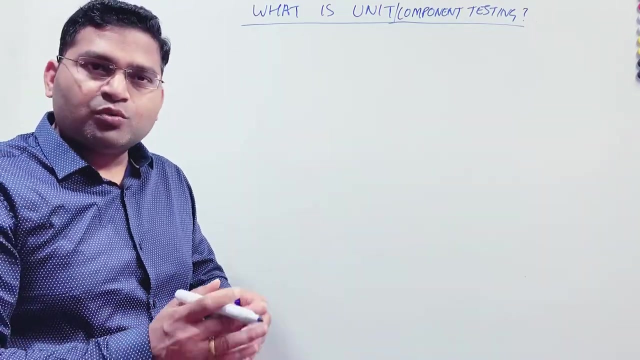 So we have understood what a unit can be in terms of car, if you broke down, break down the engine or if you break down the wheel. So put it in any sense in any of the real examples out there. just try to think about what is the smallest unit that can be tested for any product that you pick. 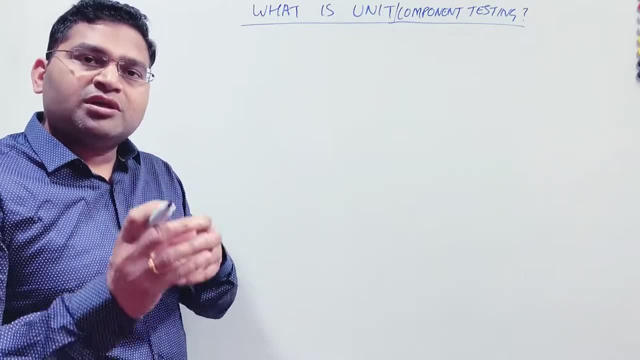 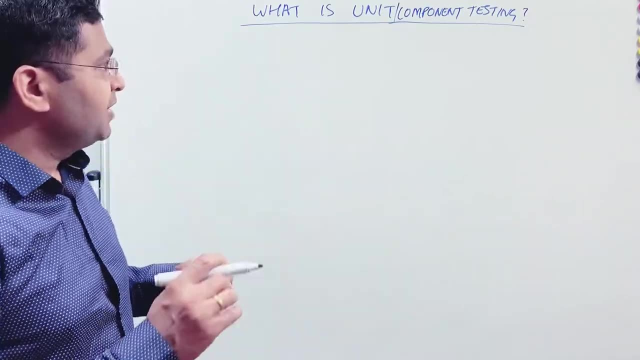 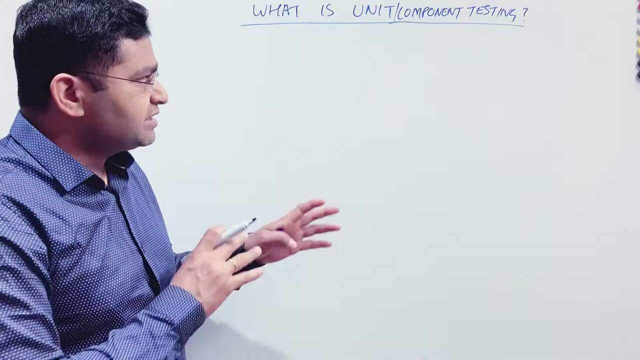 right And you will be able to understand- the smallest unit that can be tested- and that is what a unit is- Or a component is that can be tested independently. If a component cannot be tested independently, then that is not a unit, right? So if there is any sort of integration, 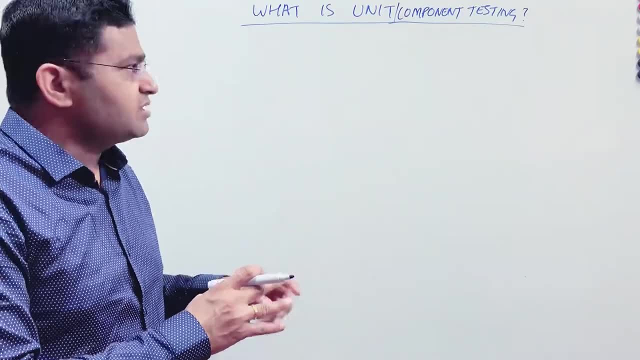 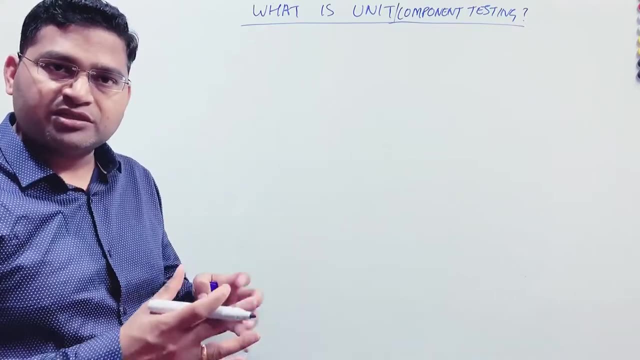 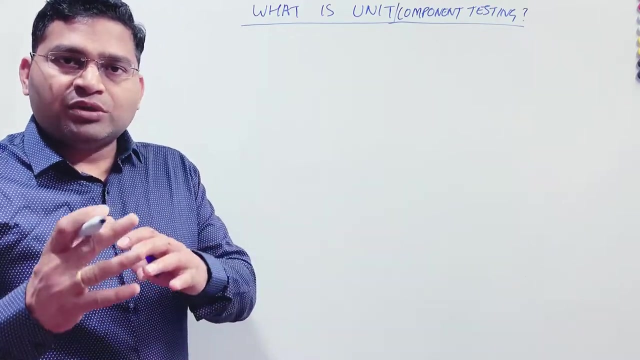 with other component, then that becomes integration testing. Now, when I try to correlate this with the software, then what could be the unit, the smallest unit in any software? So in the software world, if you're writing any program, you can say a method. 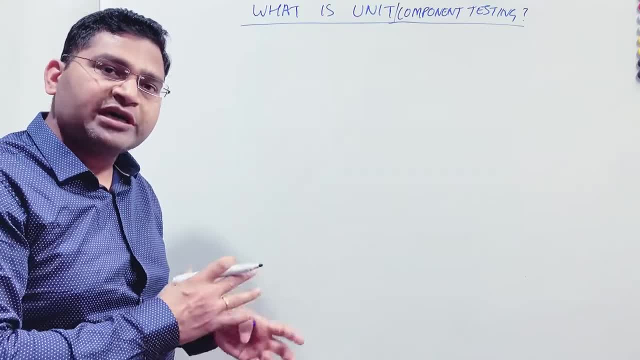 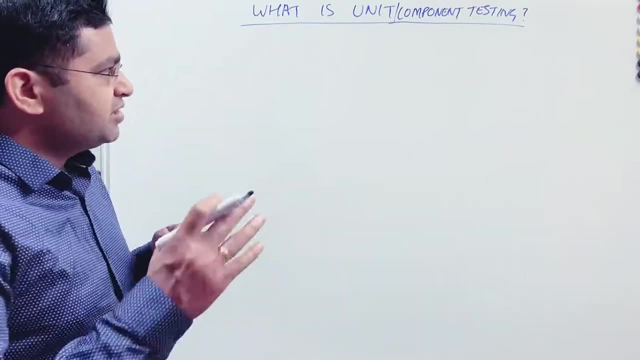 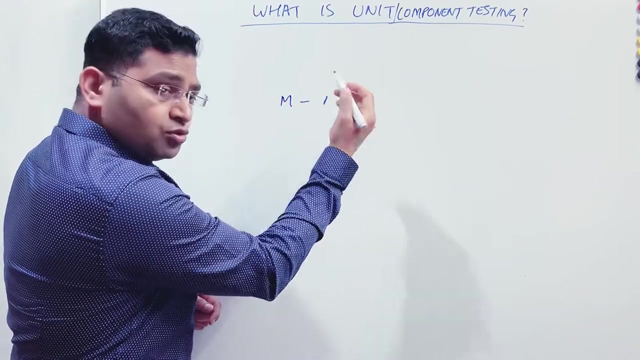 the smallest method that can be tested independently without interaction with any other. you know, component or unit is a unit in the software. Say, for example, there is a method which accepts two values, right, So which which accepts two integers? 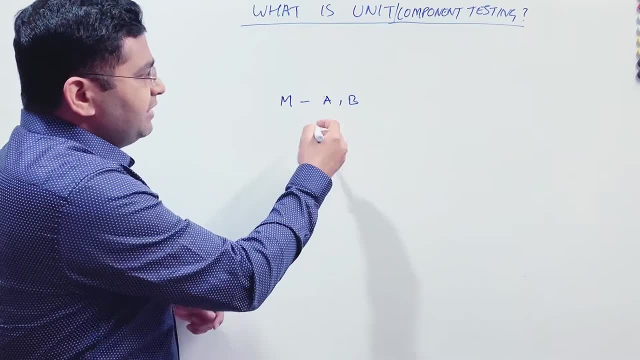 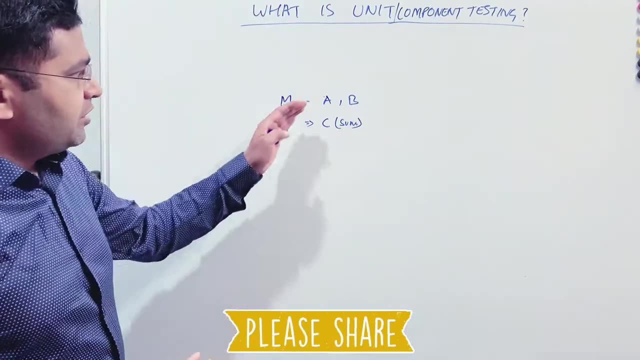 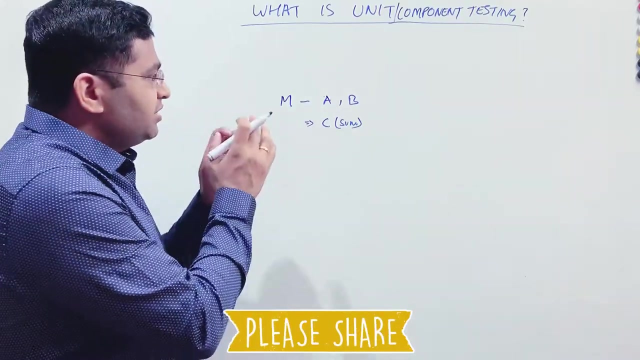 you know A and B, and then it displays the result, C, or which is the sum of two. right Now, this is what a unit will be in the software, So this is the simplest unit that you can think of. There are two numbers, So there is a method that will accept two numbers. 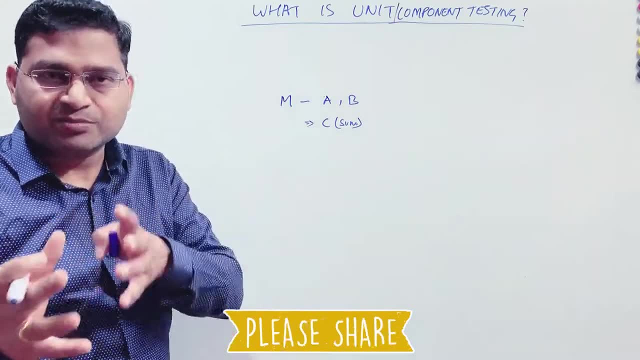 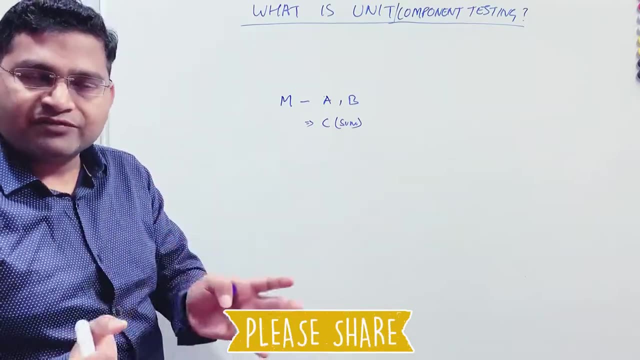 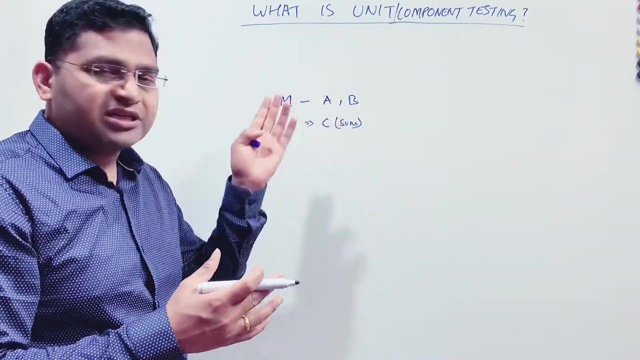 So if you write any Java program which accepts two numbers and displays the output or sum of those two numbers, this is. this method can be tested independently, right? So you can have the unit testing framework and you can write the test cases to test this particular unit. 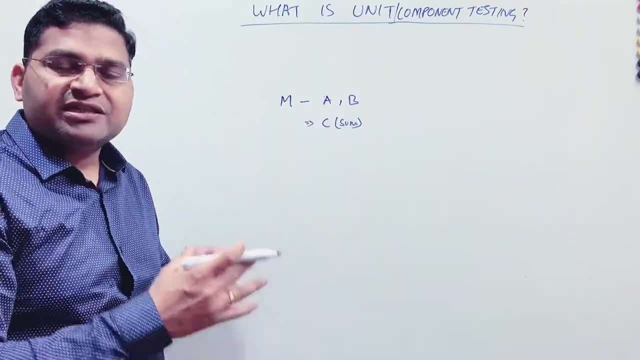 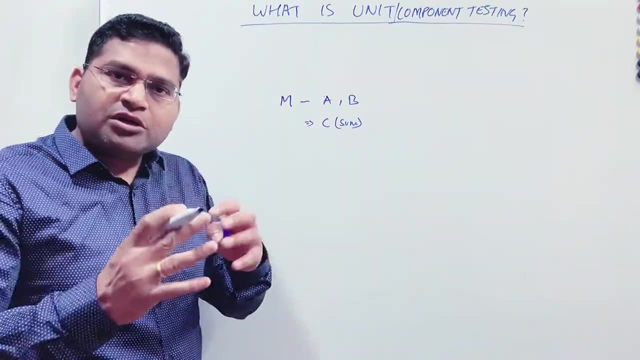 And what you're looking for now is the built in algorithm which also tests my on comma, or the method which will accept two integers and then display the sum of those two integers right. So this is what unit will be in your software. Now, if you think about the big, you know. 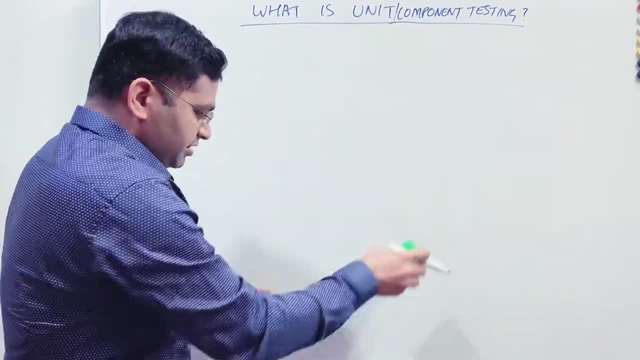 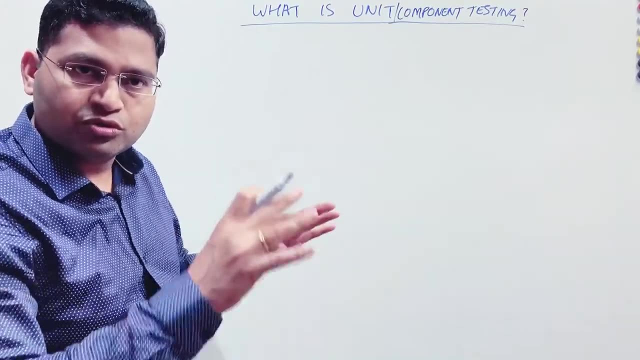 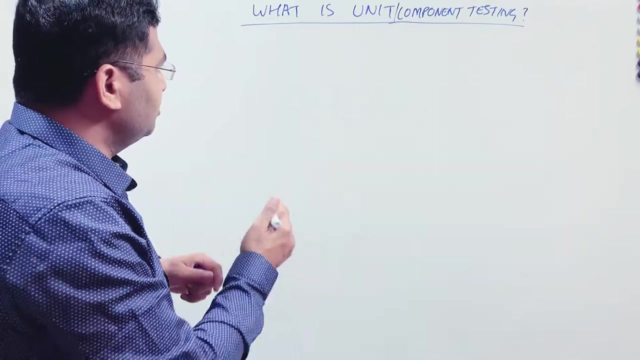 applications. we will take again the e-commerce example and in the e-commerce website, if you try to break down the overall e-commerce website into different, you know modules- right Or different- you know Application or different features that are available in the e-commerce website. 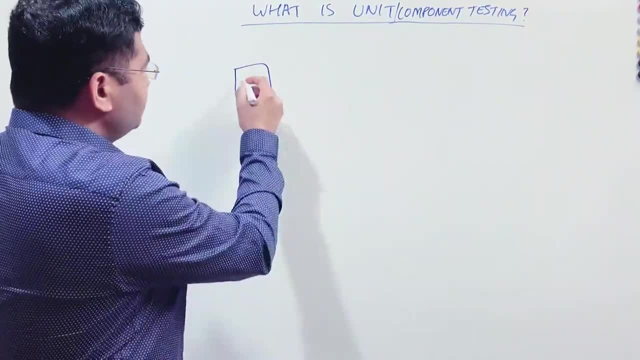 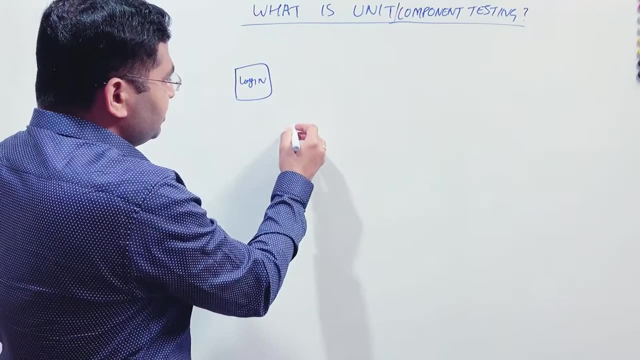 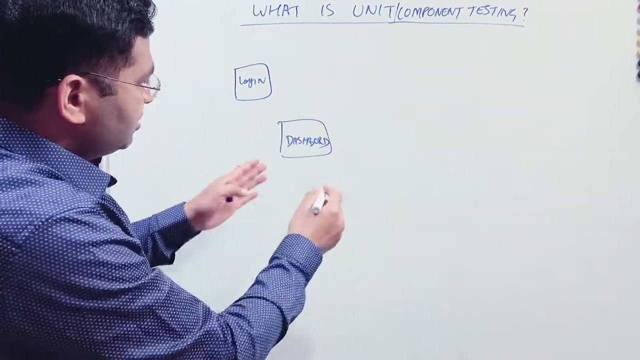 Then you will have the say: for example, the first thing is the login page, right, So high-level, you will have the login functionality, So login page. once the user logs in, then he'll be on the dashboard. alright, so dashboard Once the user is on dashboard. 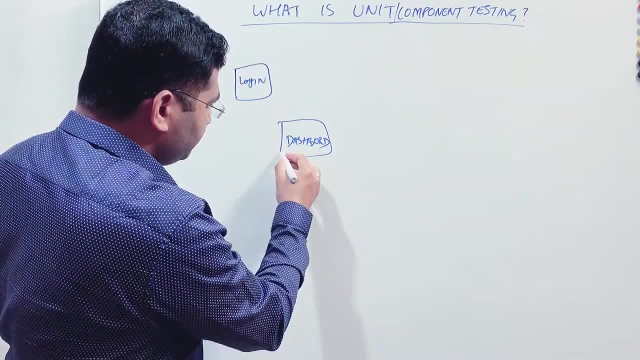 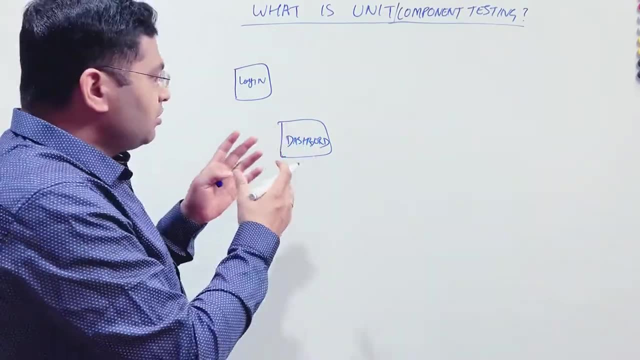 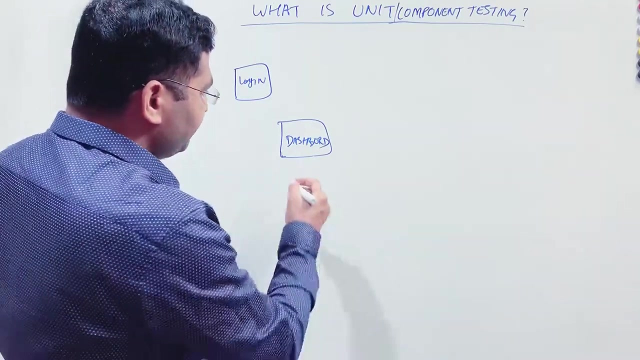 He's logged in he'll have all the you know Products that are listed there that he can actually start adding into the cart. He can add without even logging in. but with with logged in he'll have his own dashboard. He can see previous orders He can add. you know, try to buy new orders so he can add items right. 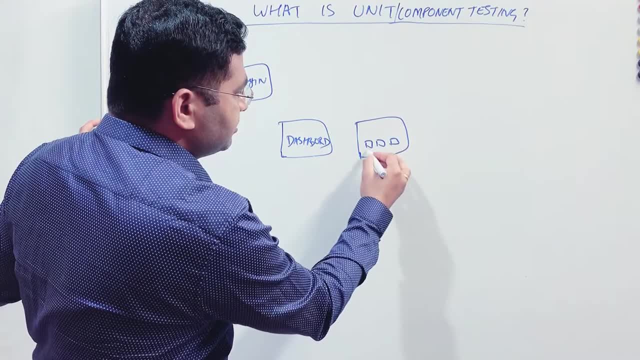 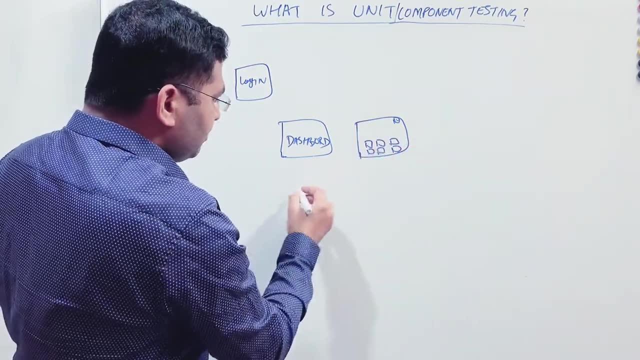 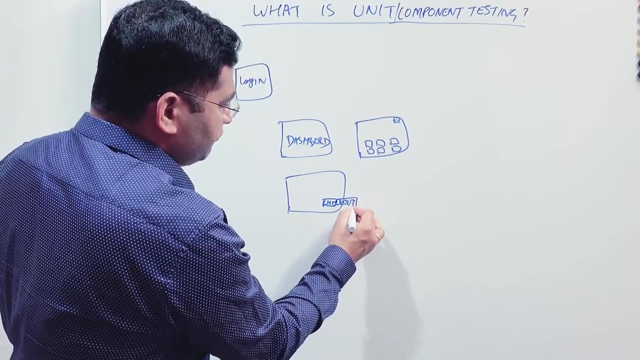 So there will be possibility to you know, Like list all the items and he can add those items in cart and cart will be visible right, So he can remove items. then he can check out, right, So there will be a checkout Functionality, So checkout button will be there. once user clicks on the checkout button It will redirect him to the payments page. 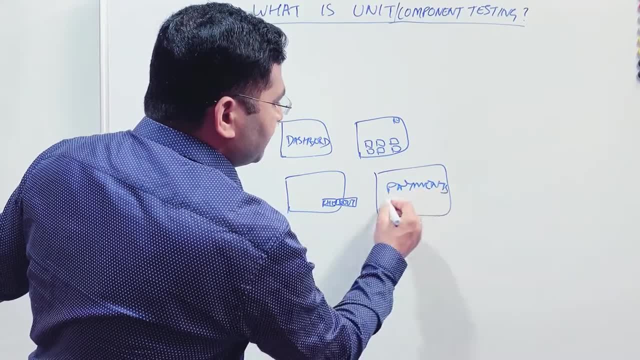 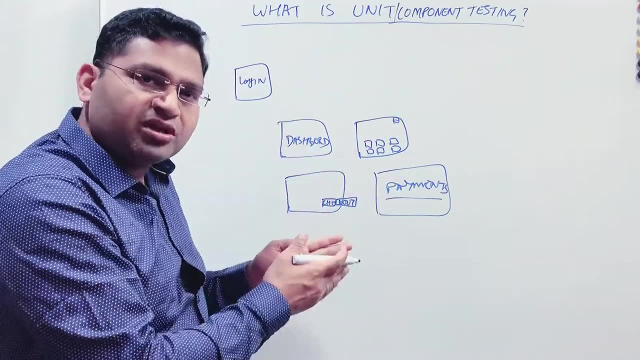 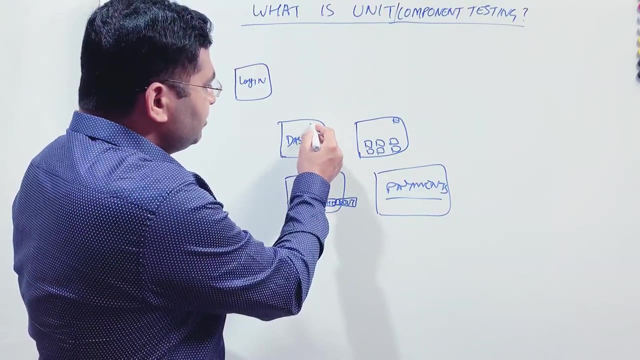 right. so these are some of the, You know, high-level features. So once he is on the payment page, he will be, you know, redirected to the payment page. he'll put the details- payment detail- and then finally make the payment and his purchase will be Successful, and then on the dashboard he will have this, his order list. 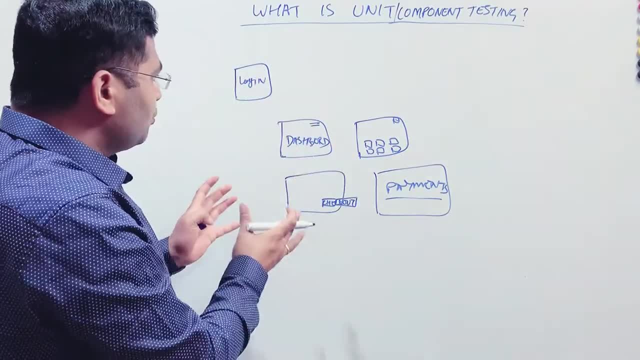 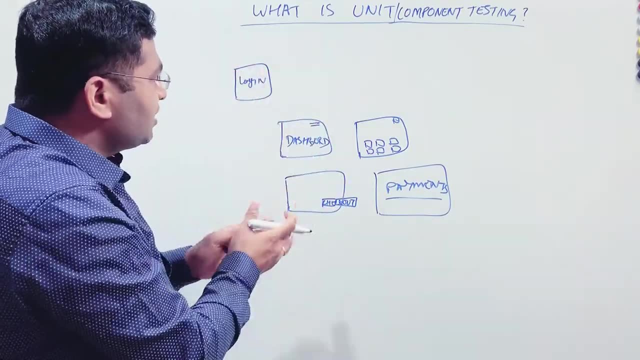 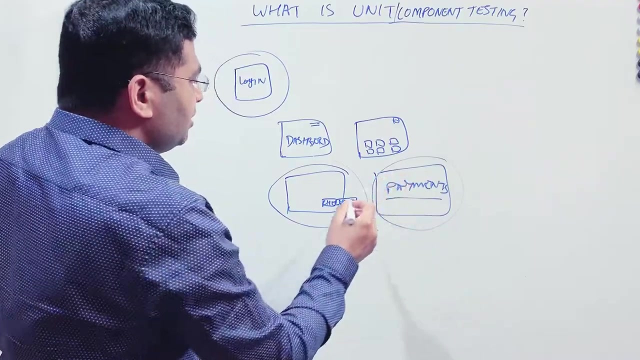 It is the order history. So this is how the Components- if you talk about the high-level components or units will, you can think of right, But actually if you try to break down even the login page or the checkout or the payments, You can still drill down a lot in terms of units or components in these you know. 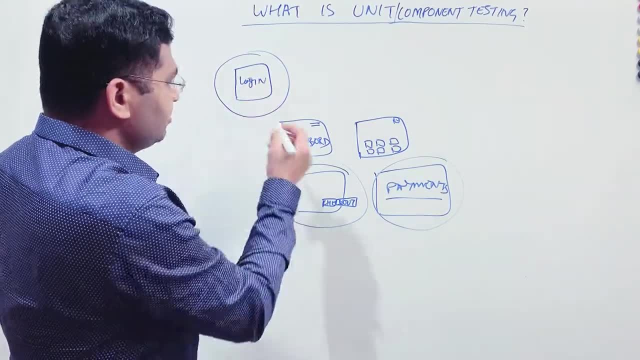 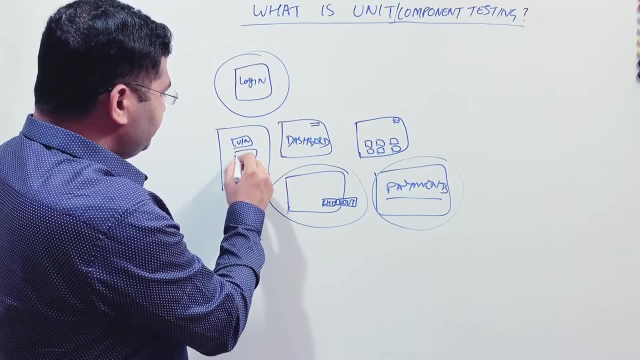 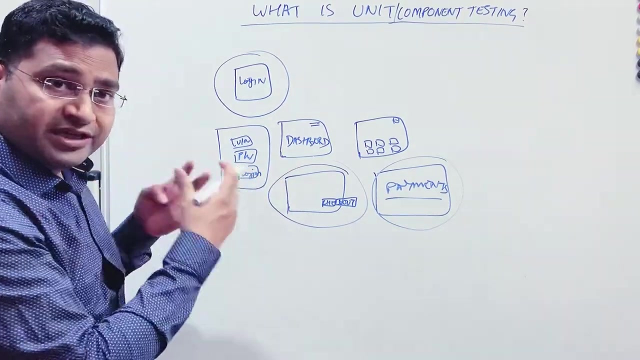 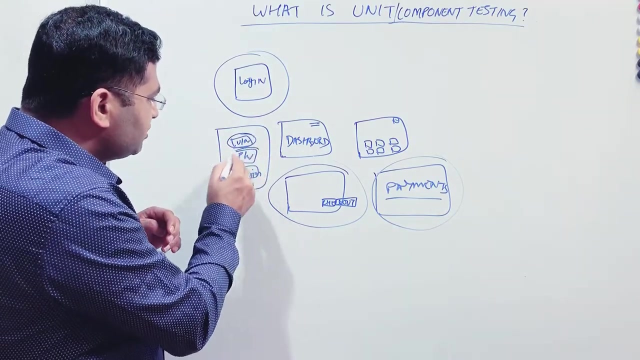 functionalities. say, for example, you know login page- right, So login page will have user username and password and then login button- right, and then there could be possibility of Logging in with Gmail, logging in with other social media accounts- right, So there will be underlying code written for each of these smaller units that you see. say, for example, there: 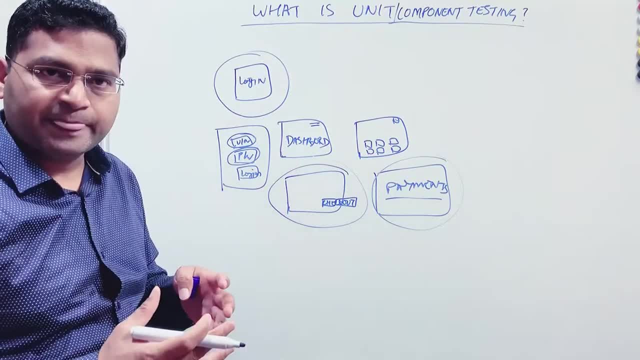 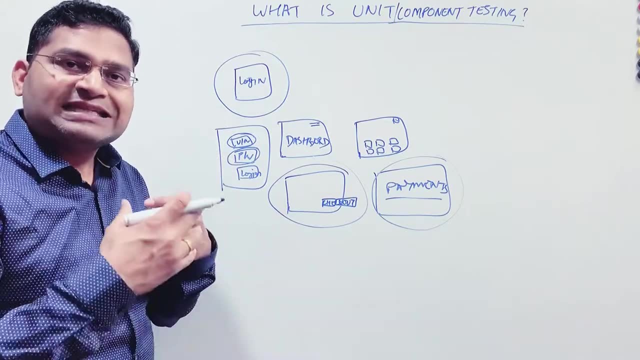 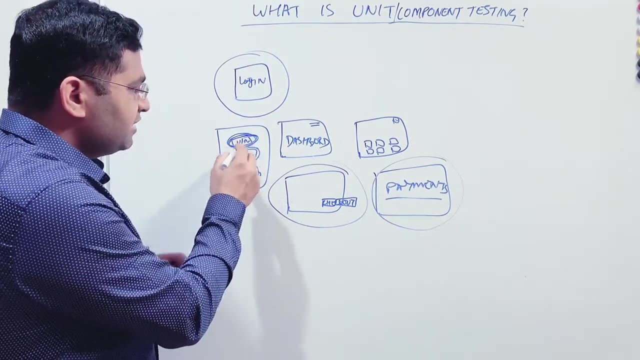 There is some logic that needs to build for the username. Okay, And if the username logic or the code written for that user Name field can be tested Standalone and is the smallest unit of code or component, then this is what you need will be right. if it is, if username field can. 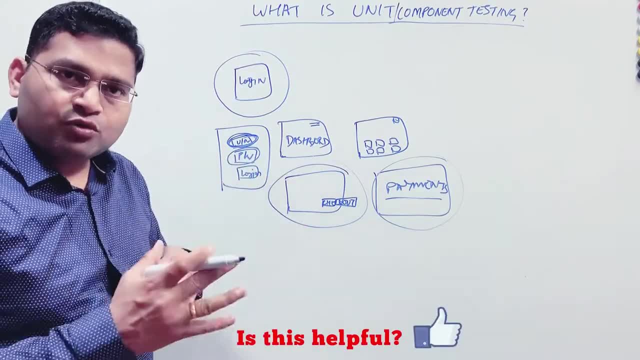 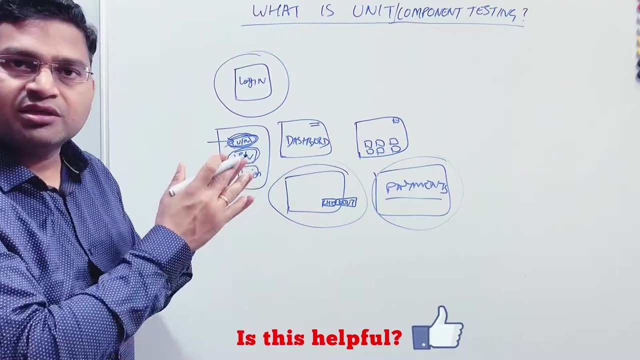 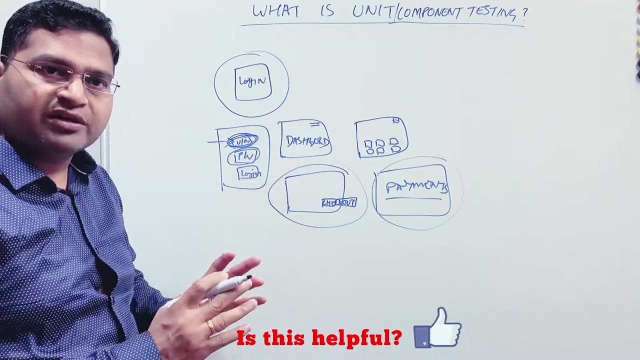 be tested independently From the code through the testing framework, for example J unit, then that's what unit is, in this particular e-commerce case, all right, so this is how you need to basically drill down into the examples, into the actual software, and Go through the smallest. 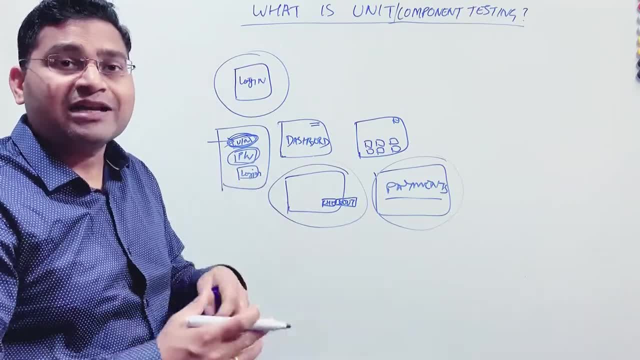 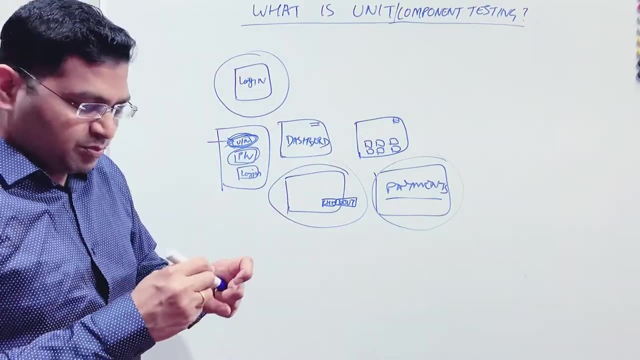 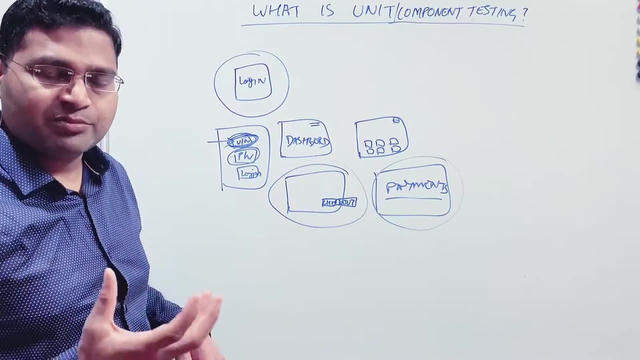 You know, understand, the smallest unit that will be possible that can be tested independently and that's what is unit or component testing, right? So the smallest testable part of the software is The unit and testing that unit, independent unit is known as unit testing in the software. now, 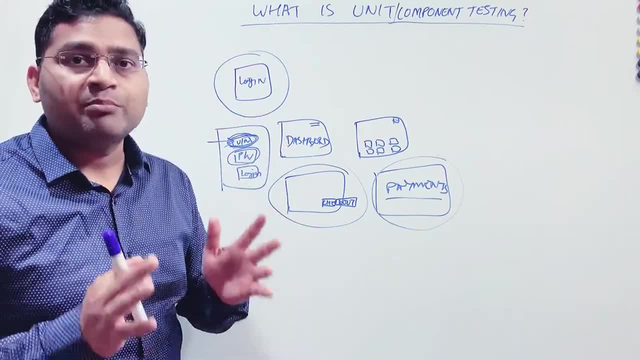 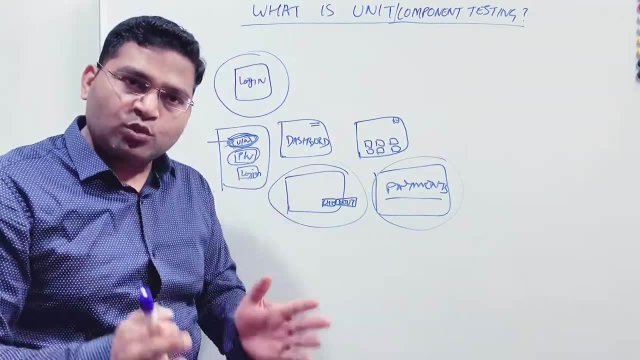 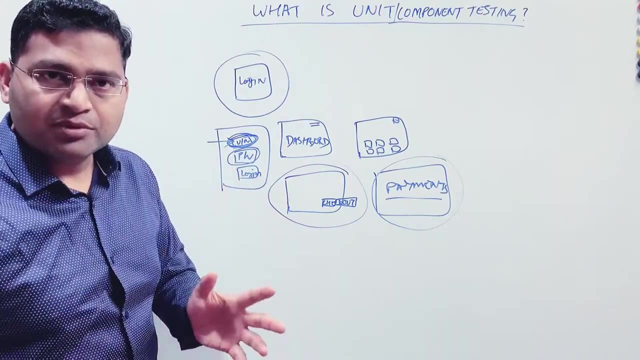 You need testing or component testing is most of the time done by developers. All right, so development team does it. but there might be possibility: if you are a white box tester or know how to Write the unit test cases, you might be required to help the development team to test. 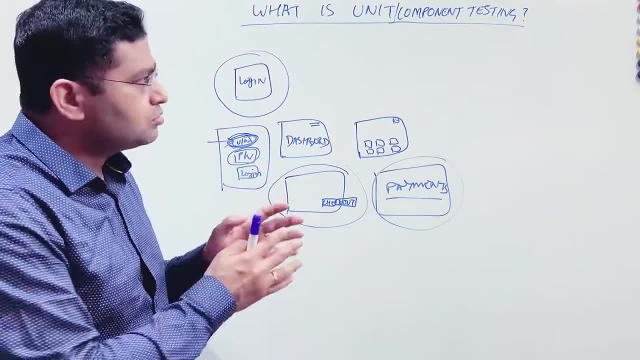 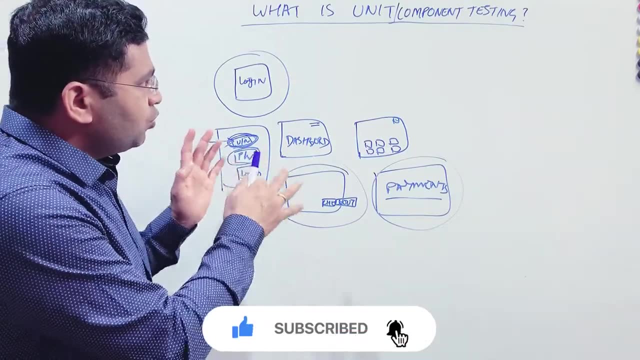 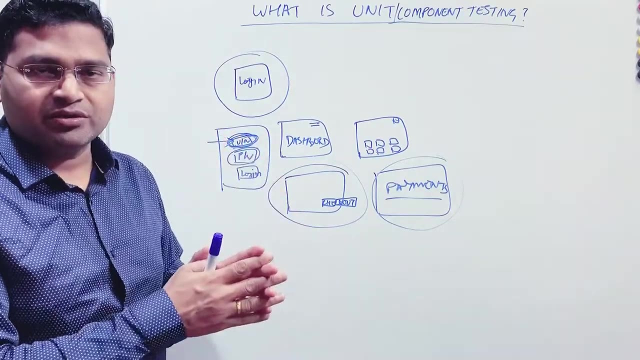 The unit or component. right, so you might be also doing the unit testing in the software development lifecycle, All right. So this is: you know what unit testing is and what is your role might be in terms of testing the unit. okay, testing the components within the SDLC. this will be.